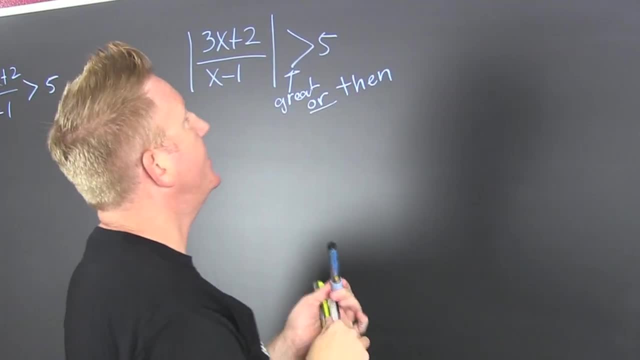 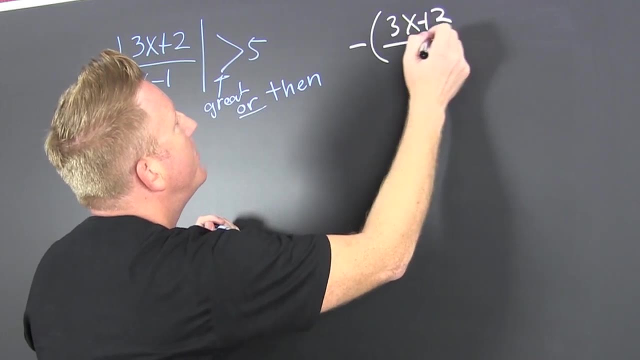 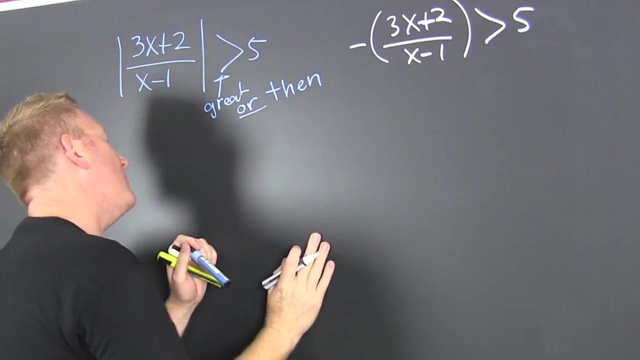 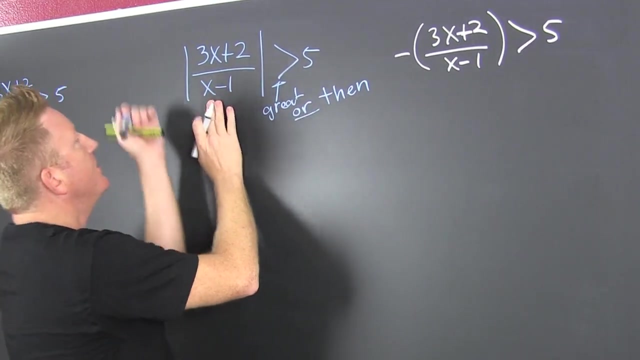 5, or the other case, the opposite of 3x plus 2, divided by x minus 1, is greater than 5.. Yeah, Okay, That's not what my book says. Alright, Multiply both sides by a minus. What I like to break it up like that. Why? Because this could be positive or this could be negative. Your book breaks it up in the: 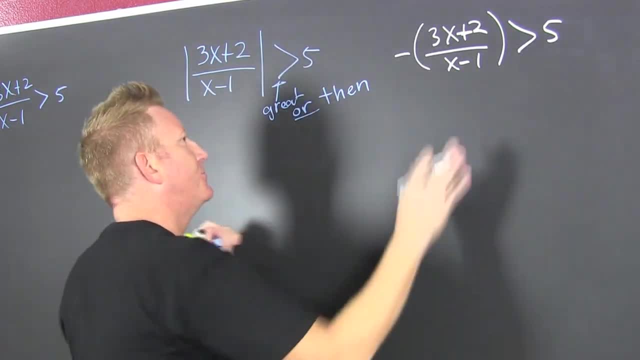 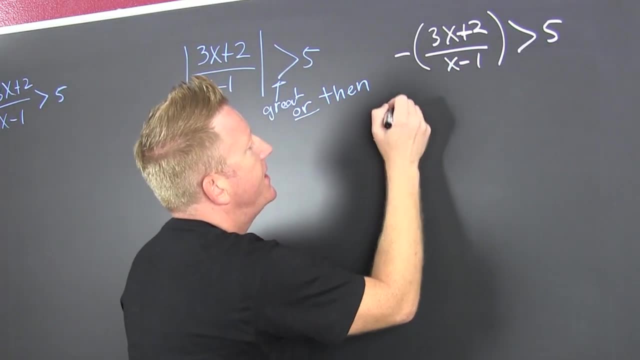 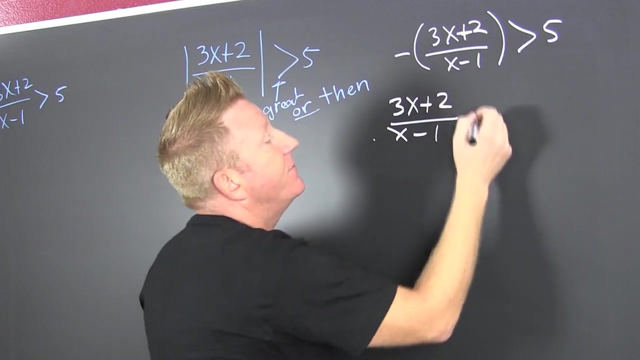 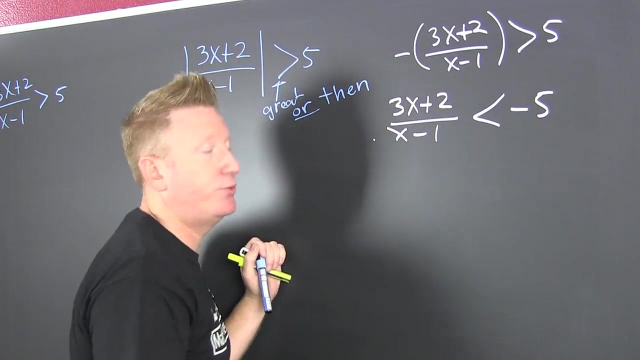 like five different cases, but all of those case could be replaced by looking at the positive and the negative. So I multiply both sides by a minus and I don't forget to flip the sign Game over, And don't forget to negate that other side over. there too. Now what We need to get it all to the left, So we see that. 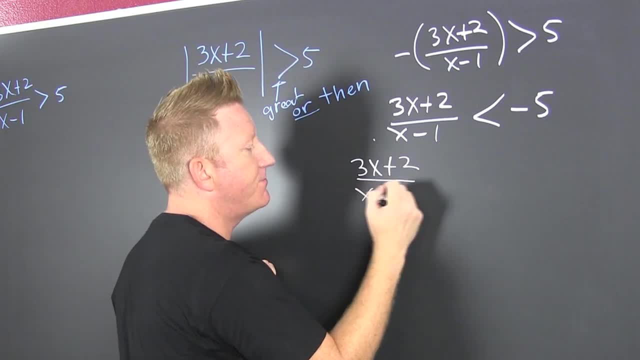 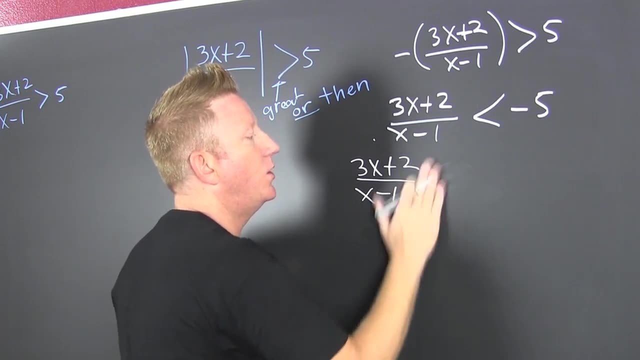 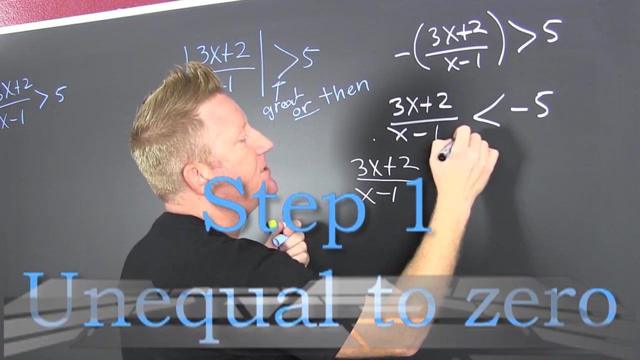 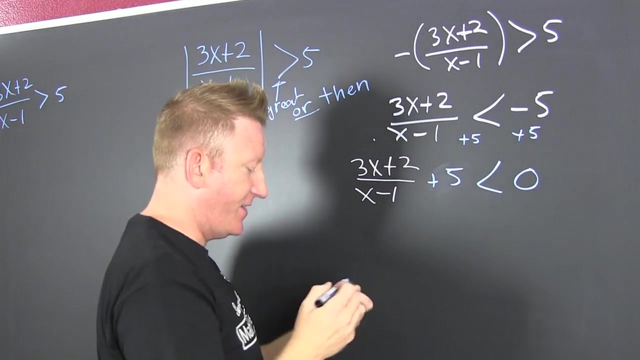 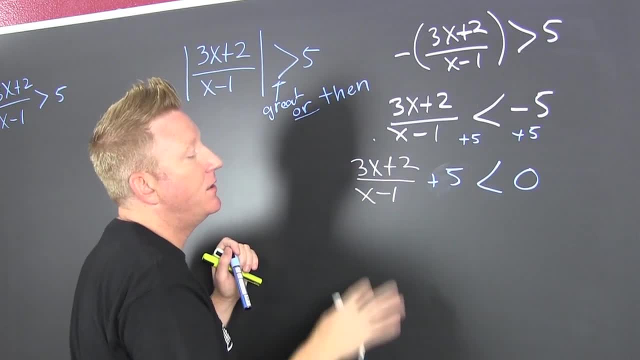 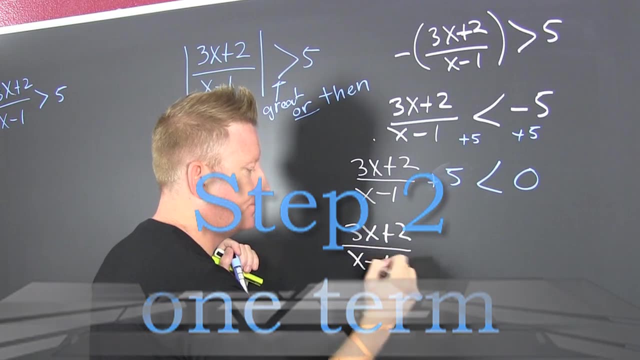 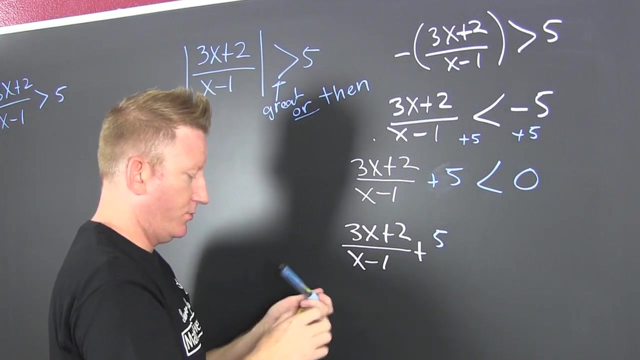 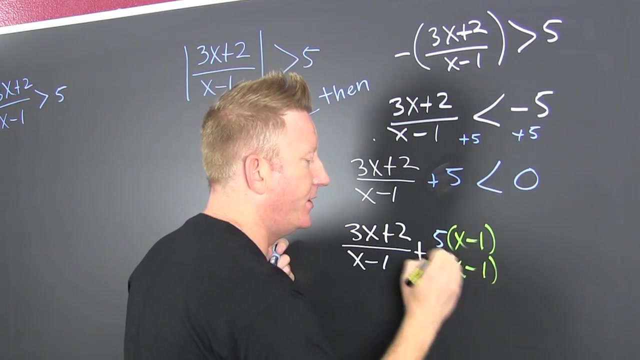 we need to multiply top and bottom by Yeah, The common denominator, Make that 5 blue. And we'll multiply that top and bottom by an x minus 1. Fun. An x minus 1. Fun. Why are you doing that? So that we can add numerators And that all needs to be smaller than. 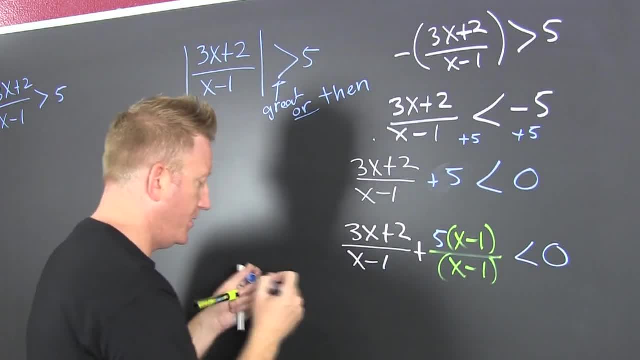 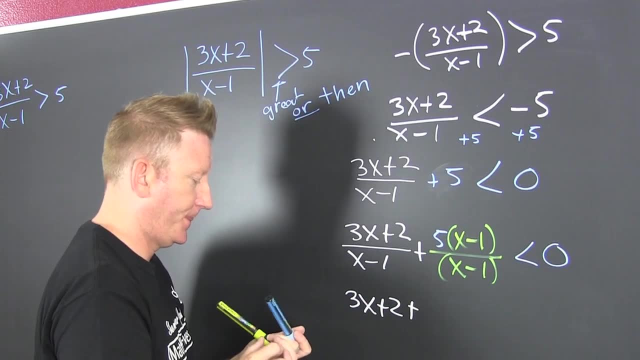 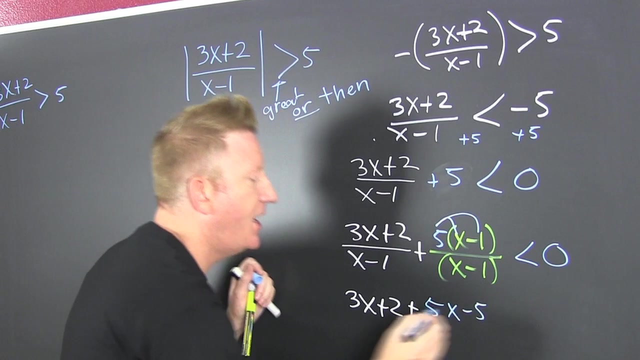 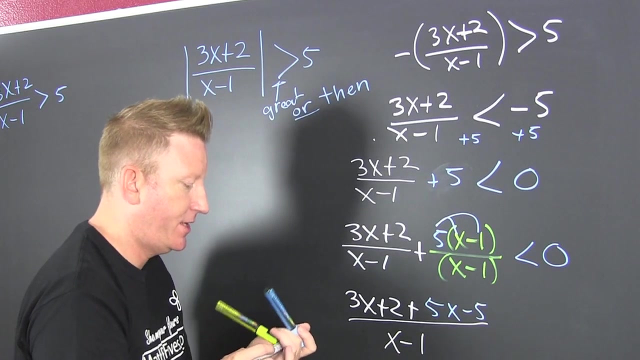 0. So now that we have that, We have, I guess it's white. That's that 3x plus that 2 plus Now 5x minus 5.. I step that skip because I'm running out of room And that's all over that common denominator: X minus 1.. Fun, And then all of that is still smaller than 0. Now I gather, collect and combine. 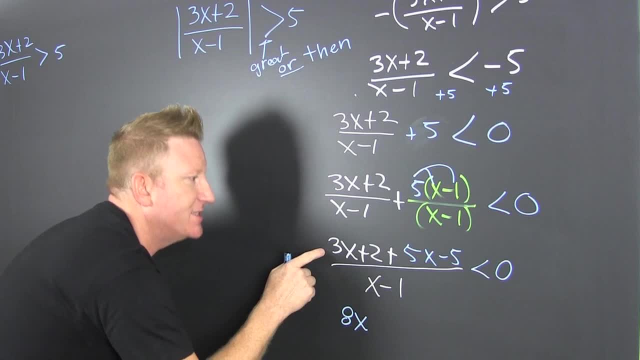 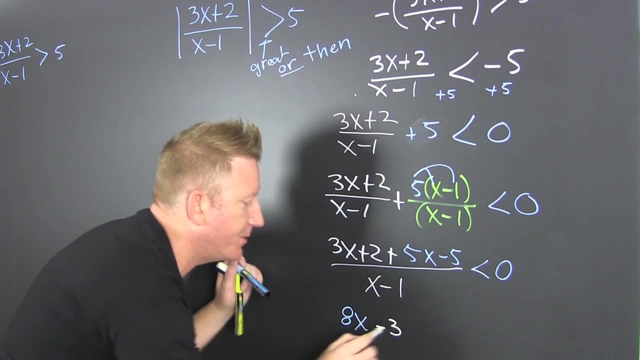 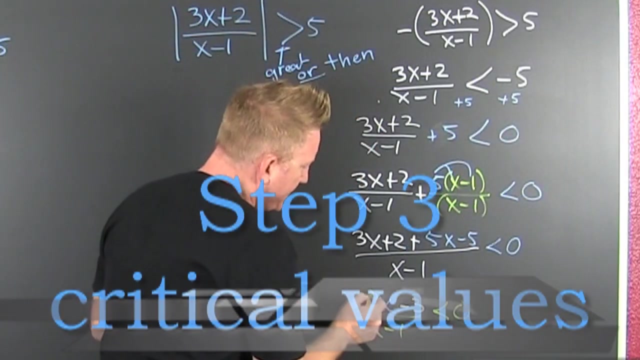 9. 8. Great Wait. A 3x and a 5x is an 8x. A 2 and a minus 5. That's going to be a minus 3. Tee hee, Tee hee. And then we see it's all over, that denominator in x minus 1. That's all still smaller than 0.. Yeah, We're over here now. All right, What makes that numerator 0?? Looks like boom. It's a 3 eighths. That's by. 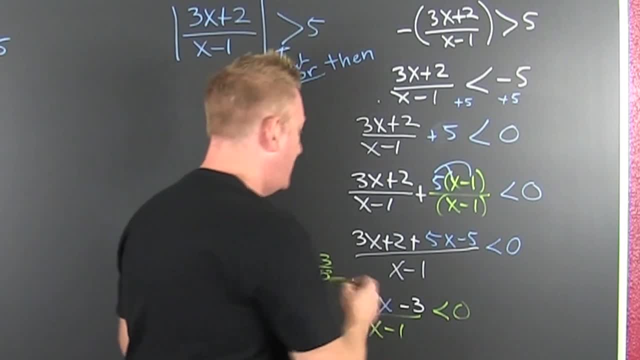 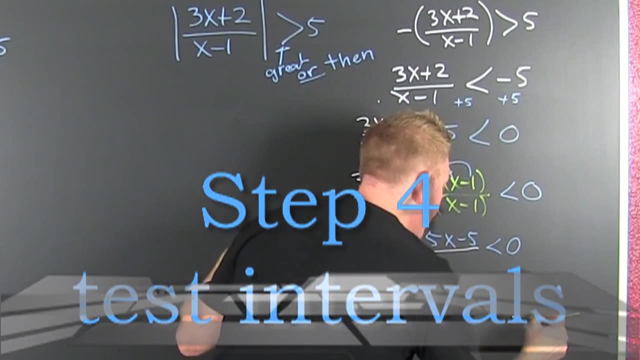 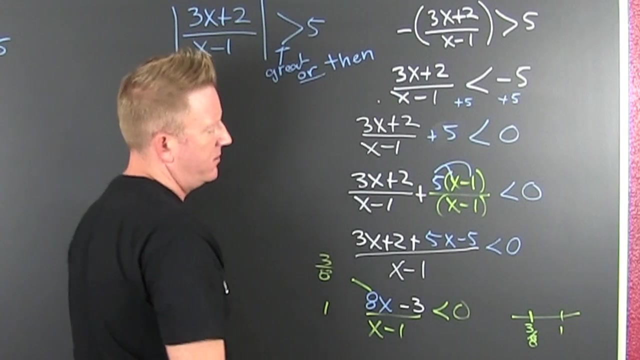 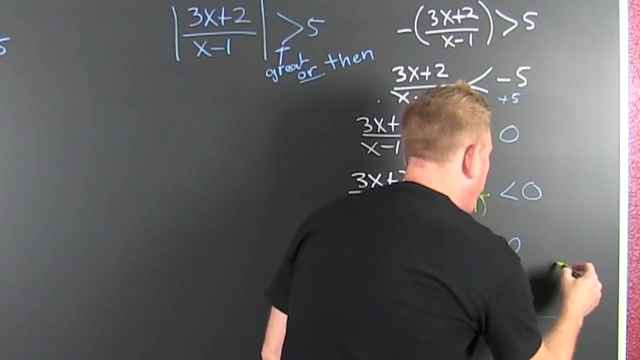 bad And then a 1. That's by bad. So those are the spots that I need to look at. That's the Yeah Positive, Yeah, Okay, Fine, Fine, Fine. 3 eighths and 1.. Fun, Now Dirty. We're checking those in The fully factored form of 8x minus 3 and x minus. 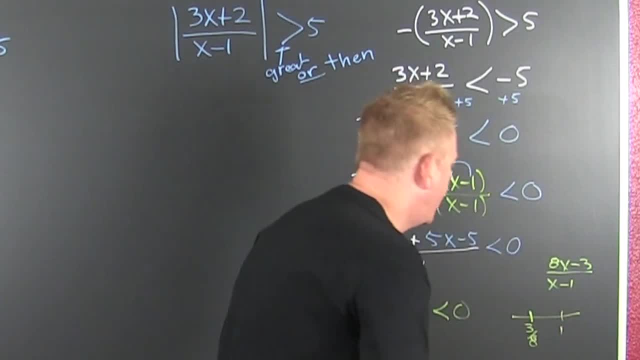 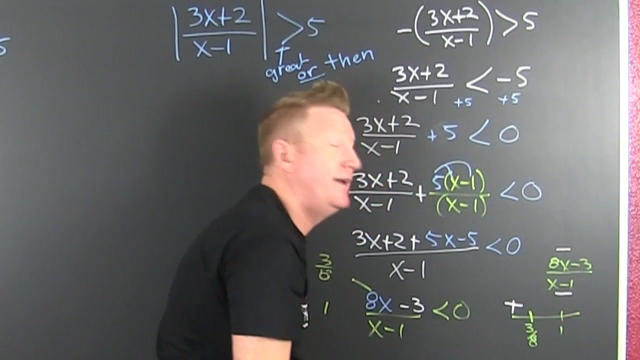 1. Are we? We're too low. All right, Shorty, I need to get a number to the left of 3 eighths. How about 0?? So we put a 0 right in here. When we put a 0 in that numerator, it's a minus 3. So it's negative. Put a 0 in that denominator: it's a minus 1. So it's negative. So the whole dang thing. a minus divided by a minus is plus. Now I need to pick a number between 3 eighths and 1.. That's the part that I'm going to need to look at. 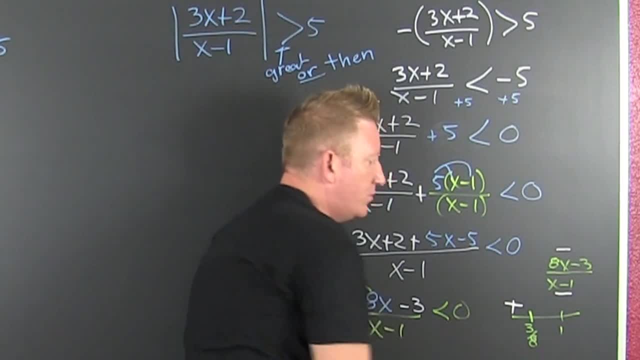 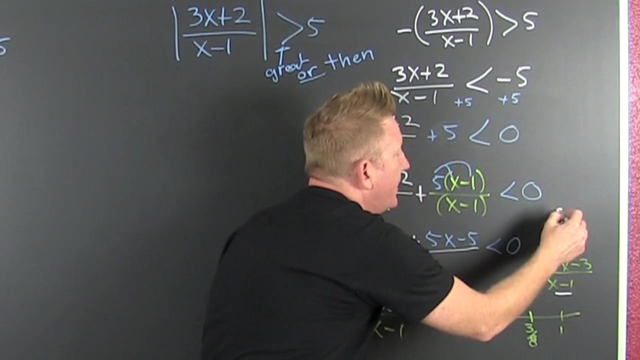 I was all like Let's go with 4 eighths Bigger than 3 eighths, Smaller than 1.. 4 eighths or 1 half. So I put 4 eighths in there. That's positive. Don't believe me. 8 times 4 eighths minus 3.. Looks like those go. It's 4 minus 3.. The dang thing is freaking positive. 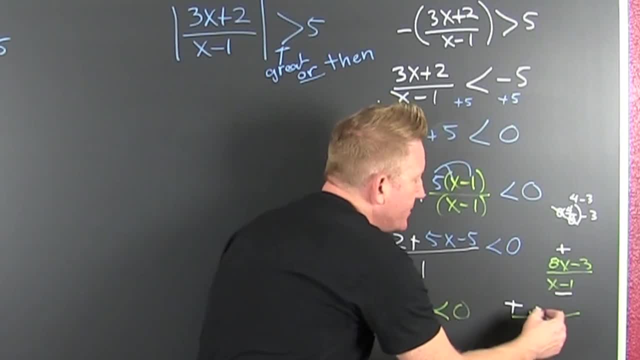 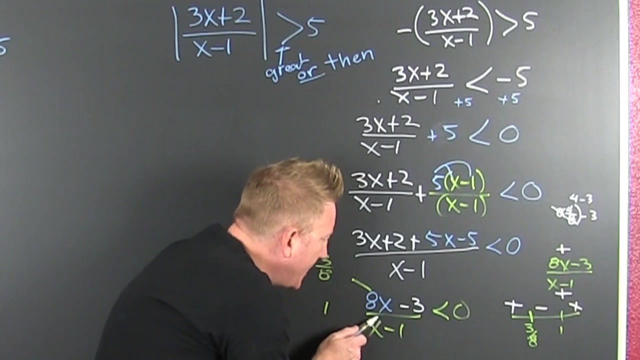 And then I put a half in there. A half minus 1 is negative, So it's negative right there. I pick a number bigger than 1.. Bigger than 1.. A million, Whatever. So 8 million minus 3 is positive And a million minus 1 is positive. A positive divided by a positive is positive. What am I looking for? I'm looking for where this is smaller than 0. The negative numbers are smaller than 0. So looks like I'm looking at 3 eighths to 1.. In that, 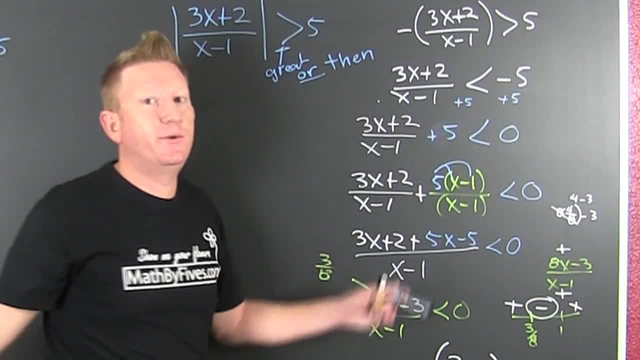 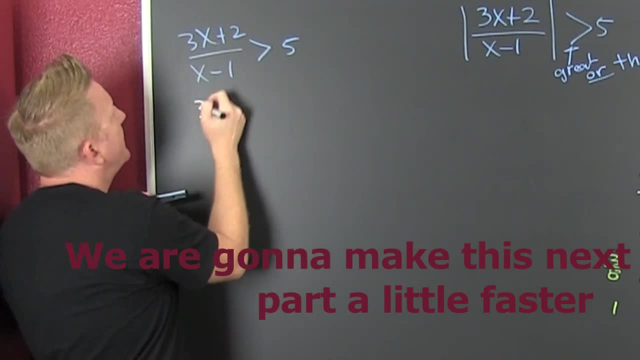 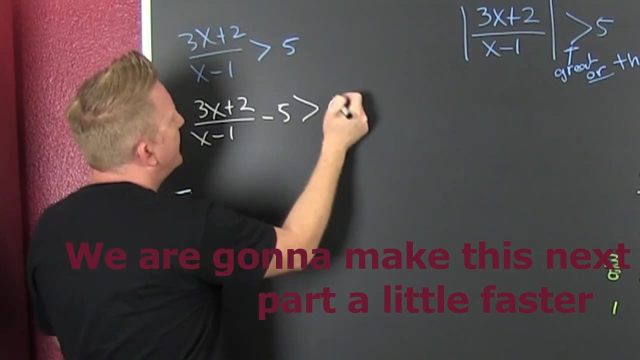 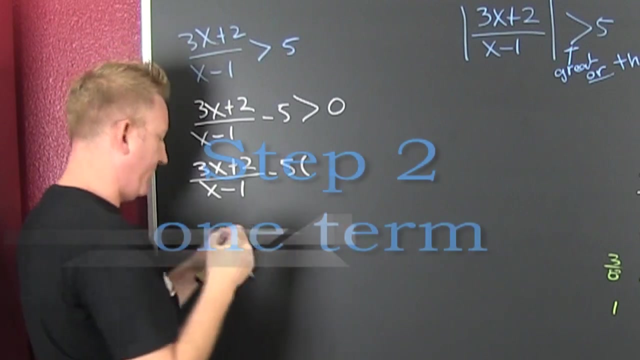 interval. That's good for that piece, But this is an or, So it's everywhere. where it's shady, You're shady. So then I put that over here. That's a 3x plus a 2 divided by an x minus a 1.. I subtract that 5 off each side and that's bigger than 0.. I gotta get that Boom, boom, boom. 3x plus 2 divided by an x minus 1 minus a. 5 times. Wait for it. Wait for it. x minus 1 divided by an x minus 1.. Fine, Let's do it. 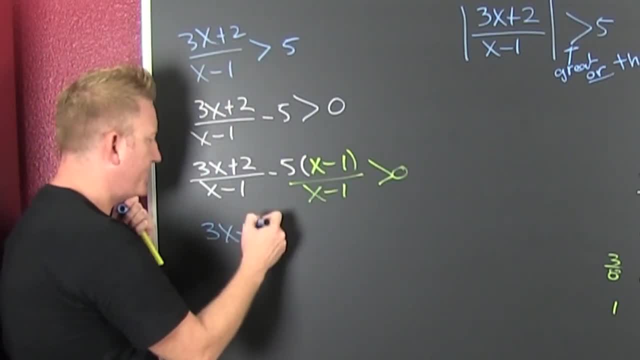 It needs to be bigger than 0.. So now that I've got a common denominator, I have to add a numerator. That's a 3x plus 2 minus a 5 times an x minus 1. now, Oh my gosh, That's. 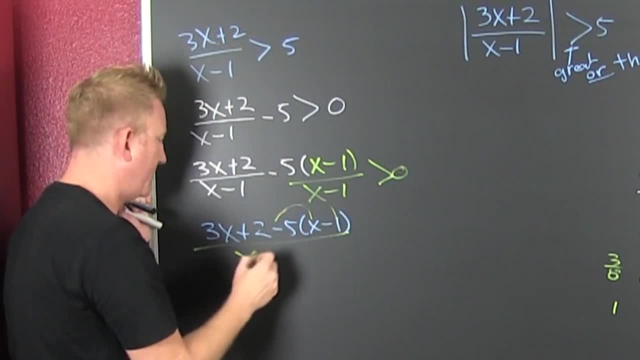 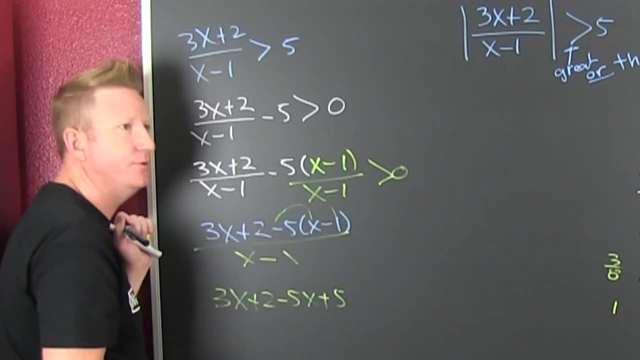 good. But here I included it Just so you don't forget to take that freaking negative here and here. But to be clear, it's still over that common denominator. Ah, It's a sideways one. So now it's a 3x plus a 2, minus a 5 plus a 5, because it goes All right. So it's. 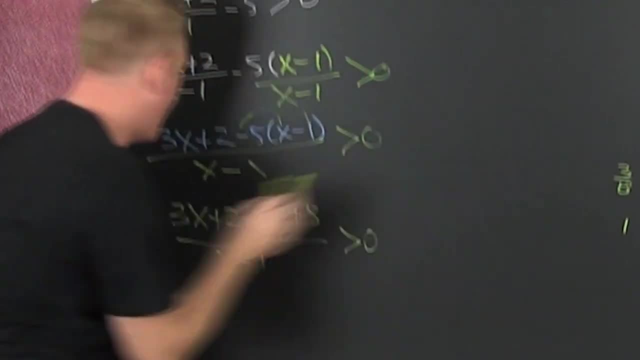 all over the common denominator x minus 1.. That's still bigger than 0.. That's still bigger than 0.. Now I finish. I've got minus 2x plus 7 divided by an x minus 1 minus a 5 plus a. 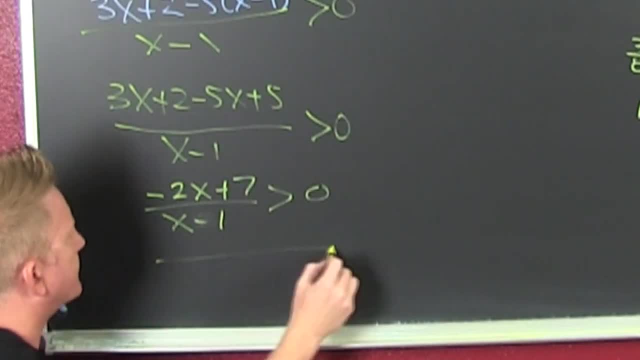 6 minus a 1.. That needs to be bigger than 0.. What are the spots on that? Looks like 7 halves and 1.. 1 is to the left. That's over here. All right, Those are the spots that. 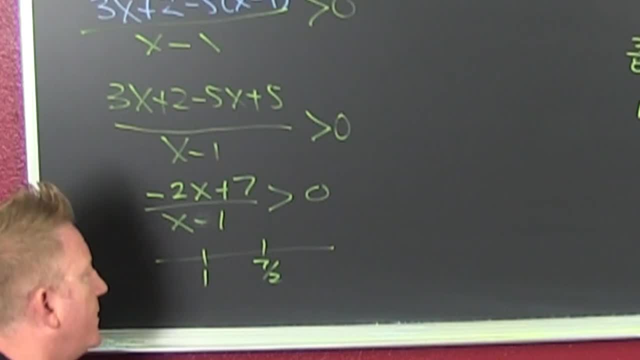 make the numerator and the denominator equal to 0. So now I need to check a number to the left of 1.. How about 0?? So I'm checking that in A minus 2x plus 7 divided by an x minus. 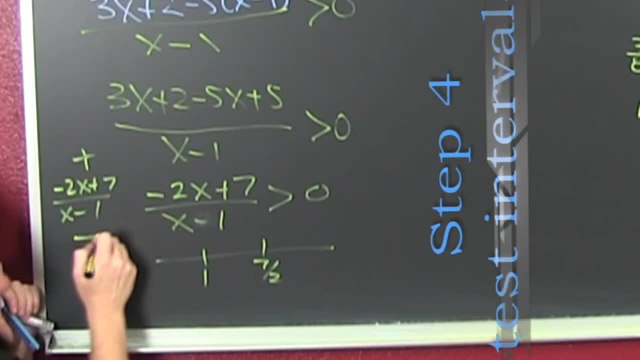 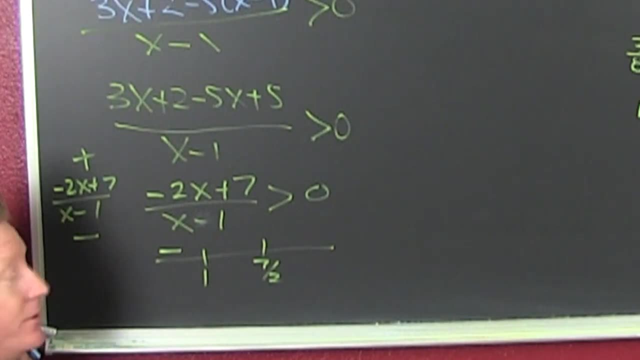 1. I put 0 in the numerator and that's a positive. 7. Yeah, I put a 0 in the denominator, That's a negative. 1. A positive divided by a negative is negative. Now I need a number in between 1 and 7 halves. How about this is? I guess I could choose 3.. 3 is in there. 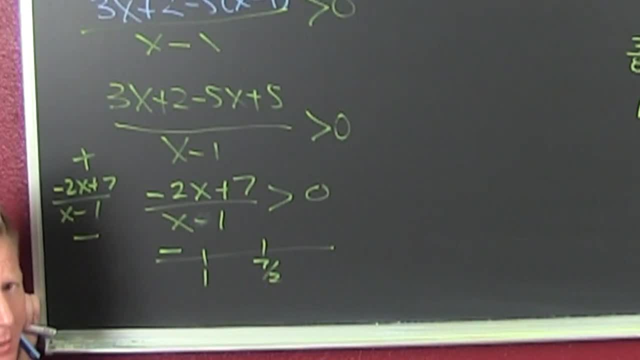 too. How do I know? Because that's why. Yeah, So any number between 1 and 3 and a half, I can plug that in there. Let's just put 2.. So I put 2 in that numerator right there. 2 times a minus 2 is a minus 8 minus. 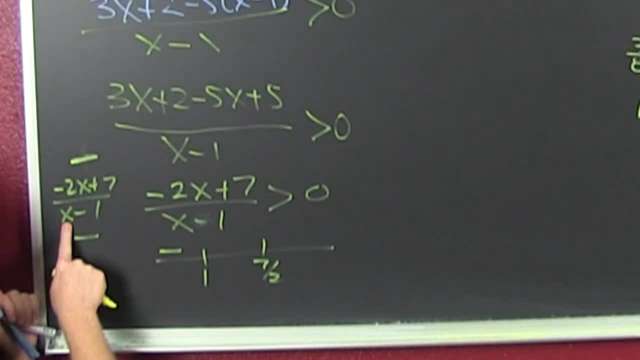 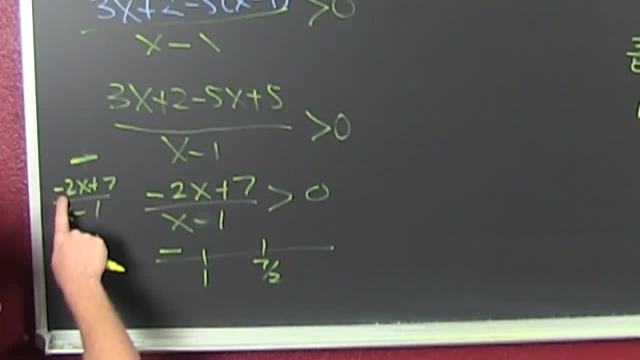 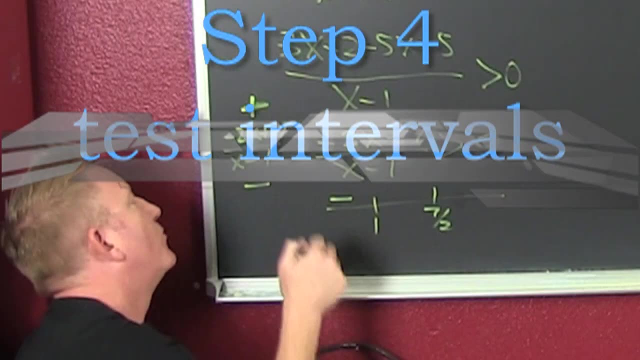 have happened? Should have. I was checking 2.. 2 times a minus 2 is a minus 4.. Sure, Minus 4 plus 7 is a positive 3.. Now I put 2 down there in the denominator 2 minus 1. 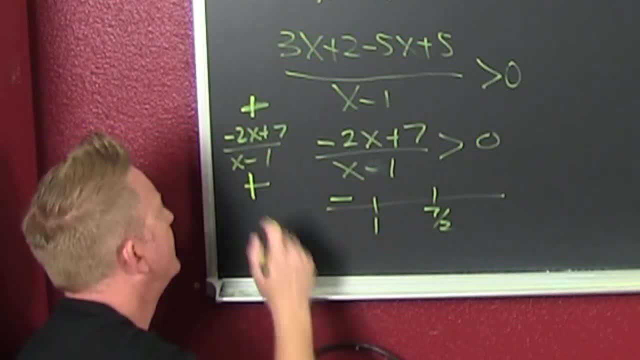 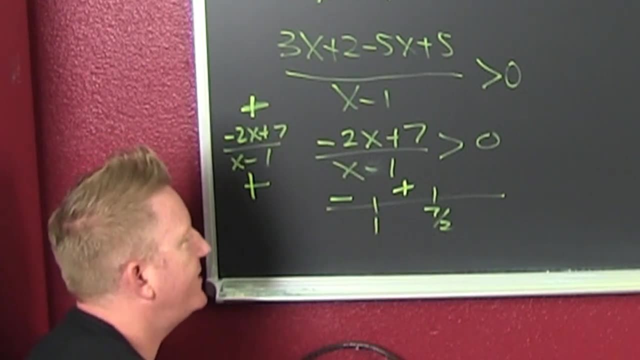 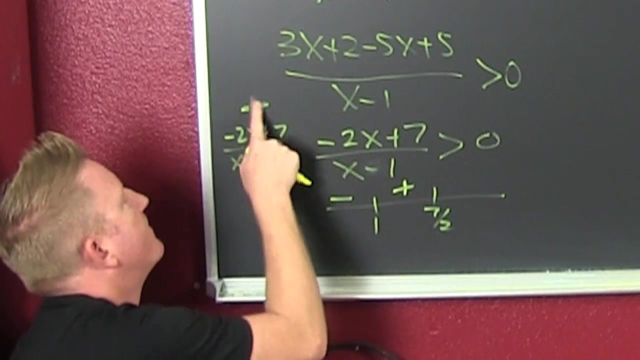 is a positive 1. Yeah, All right, Good. So a positive divided by a positive is positive. Now to the right of 7 halves. let's just put a freaking million in there, So 2 million minus 7, that's going to be negative. 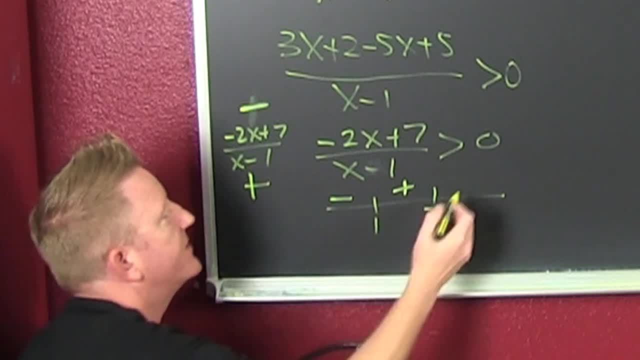 2 million minus 1 is positive, So it's negative over there. What numbers am I looking for? I'm looking for the numbers that are bigger than 0. How do I know This needs to be bigger than 0. That's where it's true, True. 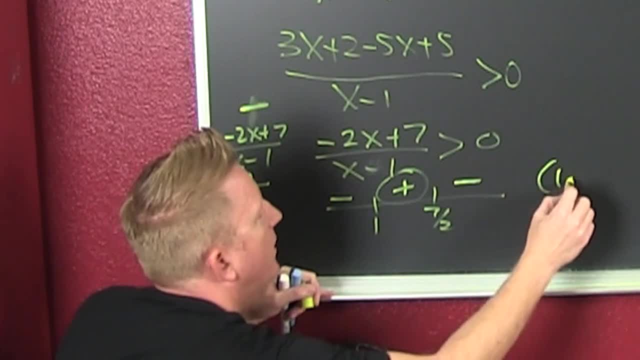 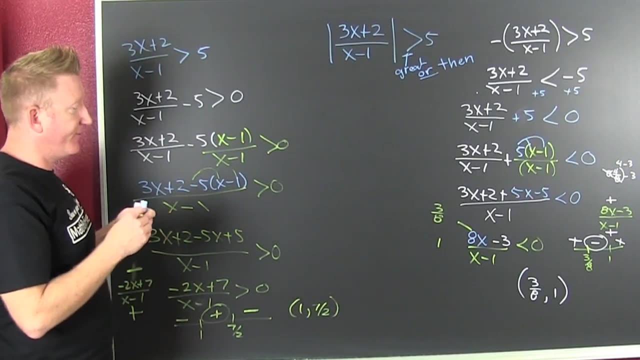 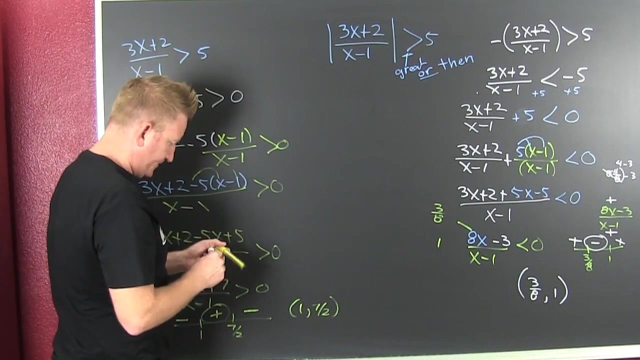 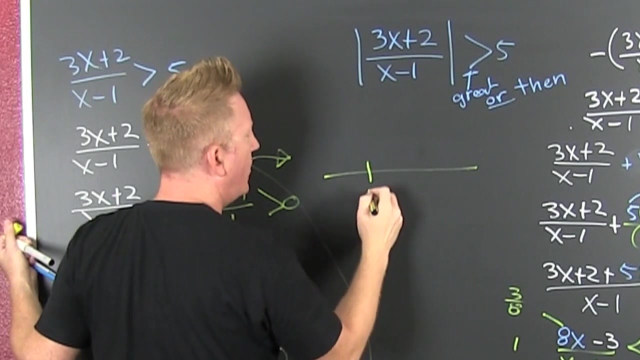 So what? These are 1 to 7 halves. Now this gets a little tricky because of the freaking fractions. So if I take this yellow group right here, Okay, yellow Yellow is from 1 to 7 halves. Good. 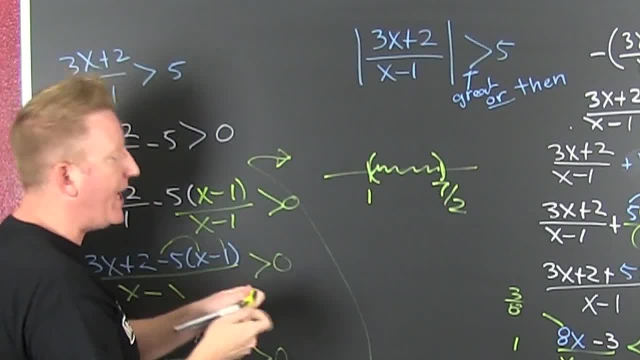 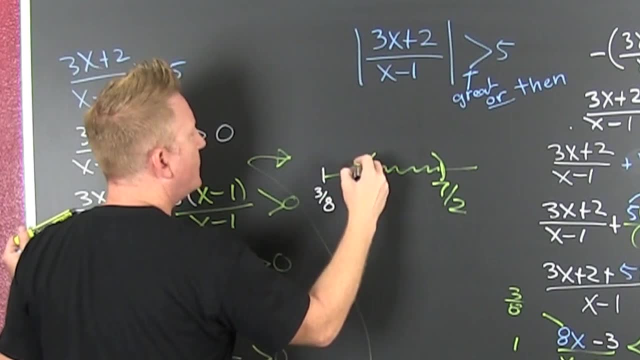 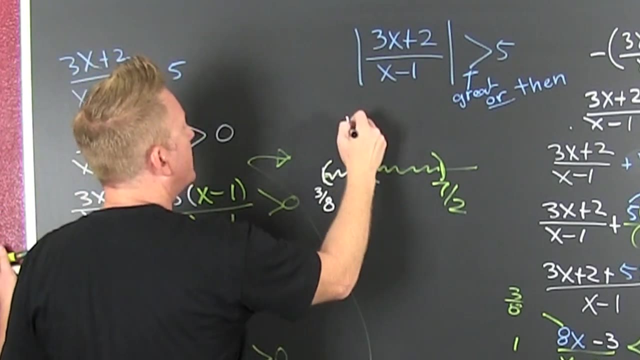 Then white is 3 eighths to 1.. So now I need to write wherever that's good: What's good people, Not 1. So 1's not good because it's not included here and it's not included there.